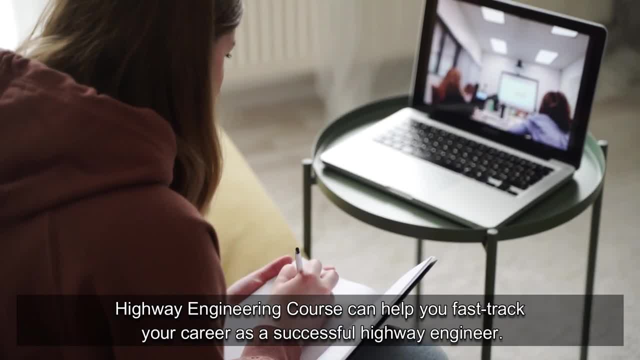 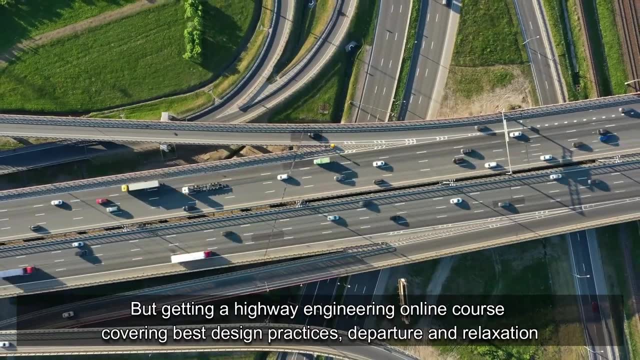 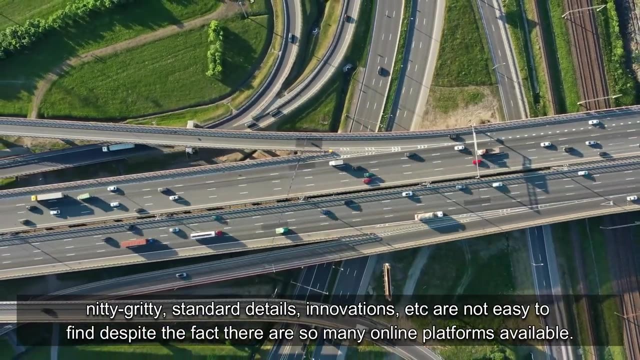 Highway engineering course can help you fast track your career as a successful highway engineer. But getting a highway engineering online course covering best design practices, departure and relaxation, nitty gritty standard details, innovations, etc. are not easy to find, despite the fact there are so many online platforms available. That's why we develop. 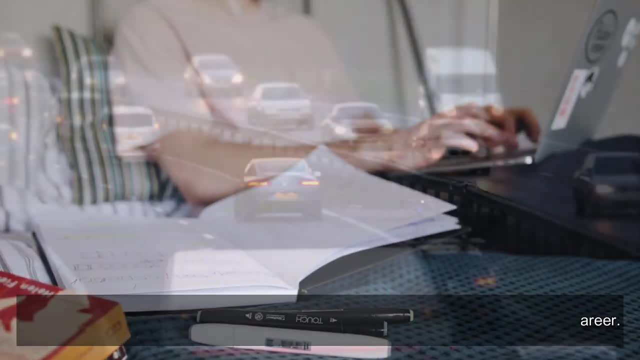 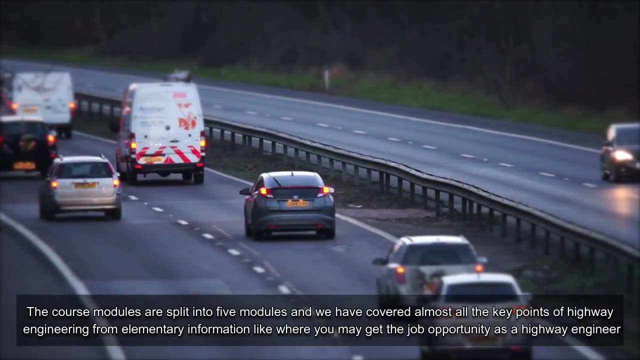 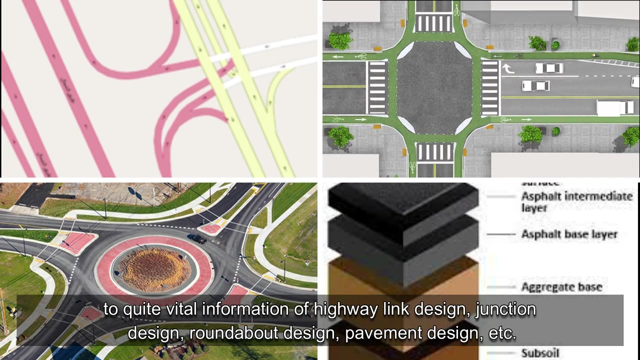 our highway engineering online course to jumpstart your career. The course modules are split into five modules and we have covered almost all the key points of highway engineering: from elementary information, like where you may get the job opportunity as a highway engineer, to quite vital information of highway link design, junction design, roundabout design, pavement design, etc. 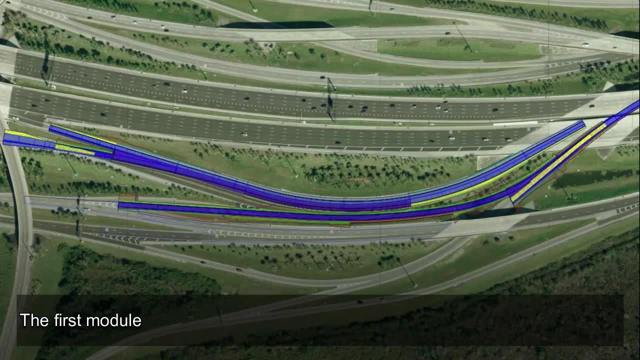 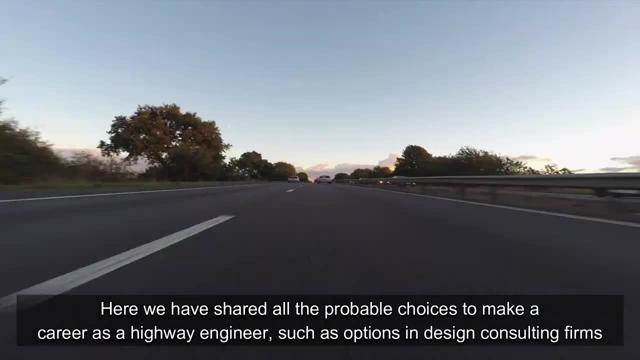 Module 1: Highway Engineering and Highway Design. The first module commences with key industries of highway engineering sectors. Here we have shared all the probable choices to make a career as a highway engineer, such as options and design consulting firms, highway engineers and highway engineers. 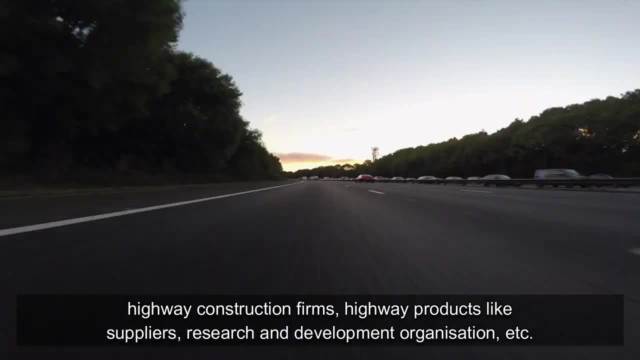 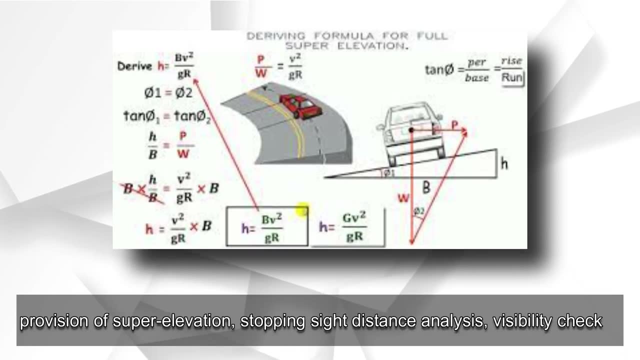 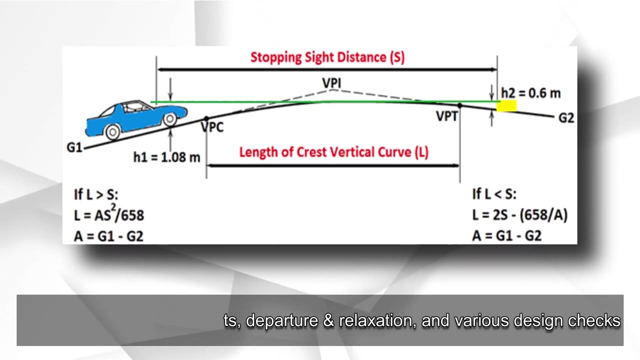 Construction firms, highway products like suppliers, research and development organization, etc. Here we covered horizontal alignment design, vertical profile design, provision of super elevation, stopping site, distance analysis, visibility checks, verge widening requirements, departure and relaxation and various design checks. Also covered curbs, footways, verges. 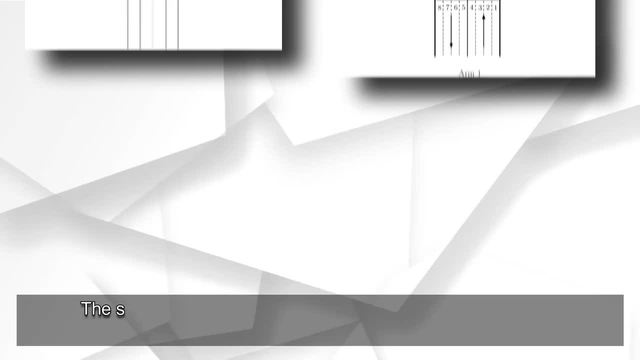 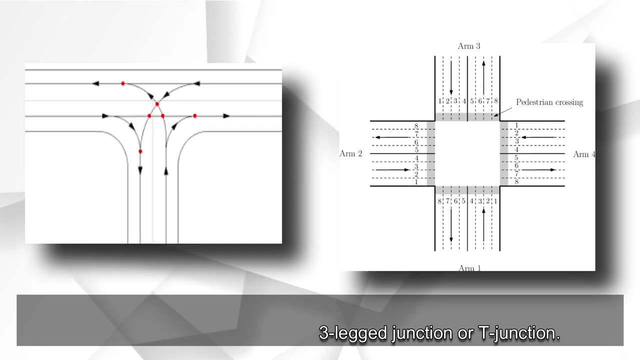 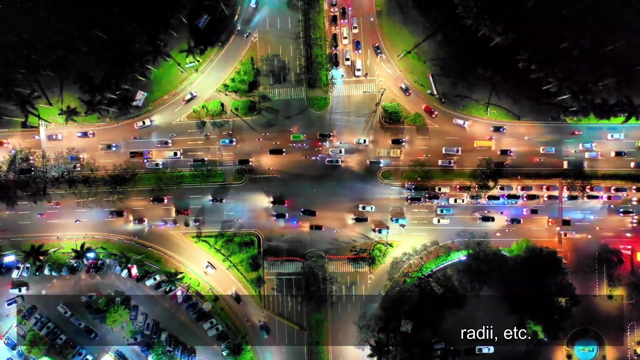 and earthwork development. Module 2: Junction Design. The second module covers the design process of the junction: design of a four-legged junction, Three-legged junction or T-junction. The module demonstrates the process of developing all the road channels: central, median, corner, radii, etc. Once a 2D road junction layout is developed. 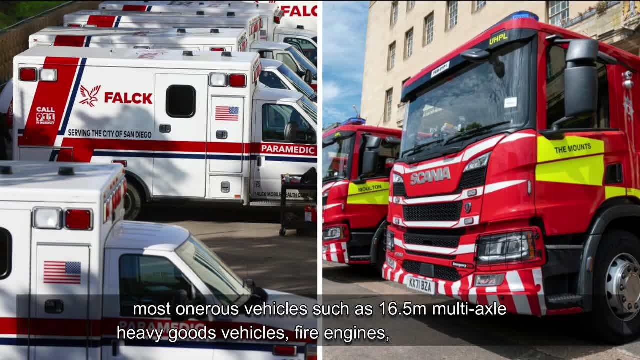 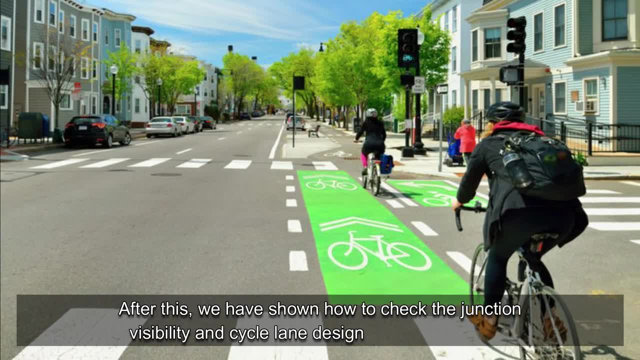 swept path analysis is carried out for most onerous vehicles, such as 16.5 meters multi-axle heavy goods vehicles, fire engines, ambulances, etc. After this, we have shown how to check the junction visibility and cycle lane design across the junction. It is recommended design the junction. 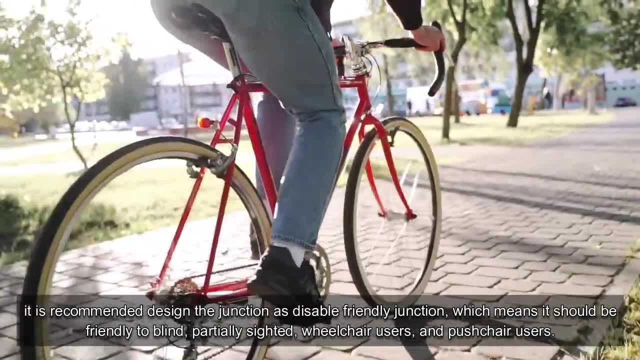 as disabled for the road. After this, we have shown how to check the junction visibility and cycle lane design across the junction. It is recommended design the junction as disabled for the road. three-leggedurofriendly junction, which means it should be friendly to blind, partially sighted, wheelchair users and. 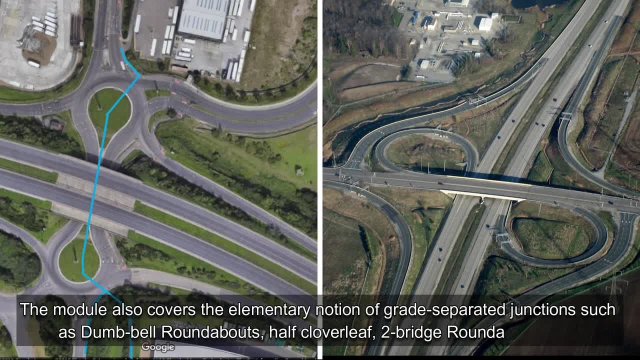 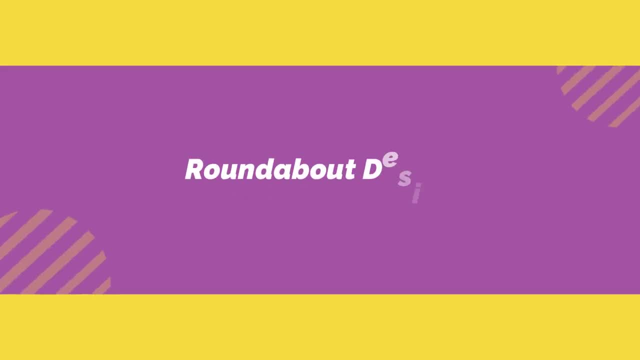 park, australia. suspension users. The module also covers the elementary notion of grade- Separated Junctions, such as Dumbbell roundabouts, half cloverleaf bridge roundabouts, eg. Module 3: Roundabout Design. The third module explains the detailed design process of roundabout design.